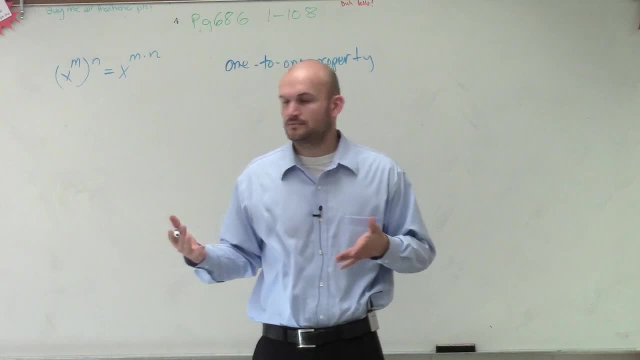 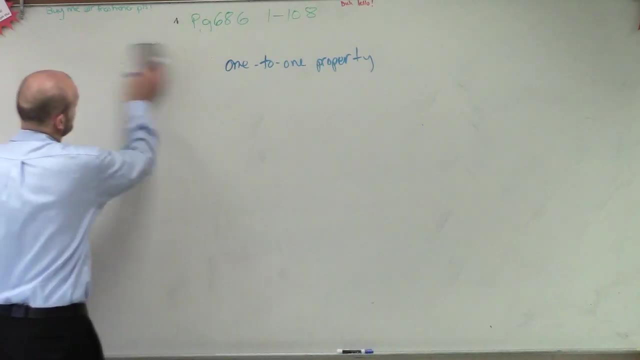 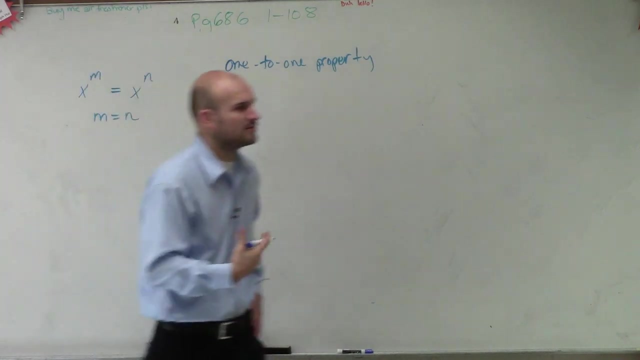 logarithm in exponential form, right? Okay, So so far we talked about our one-to-one property, for we talked about exponential form. is x to the m equals, or x to the m equals, x to the n, then m equals n, right, You could use whatever variable. you could use a and. 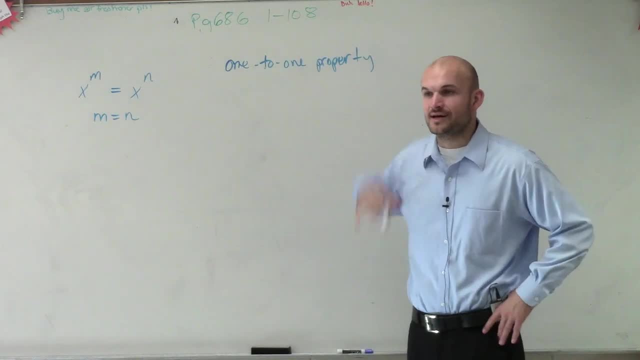 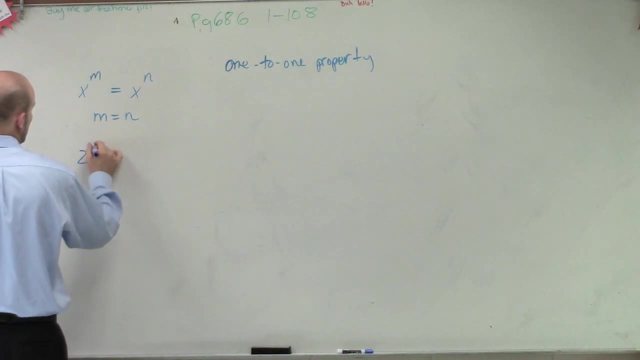 b, like I did before. but you guys need to understand that if you have the same basis, then the exponents going to be equal to each other And I proved this by doing this logarithm: Two to the x equals two to the fifth x has to equal five, right, And that makes sense. when you kind 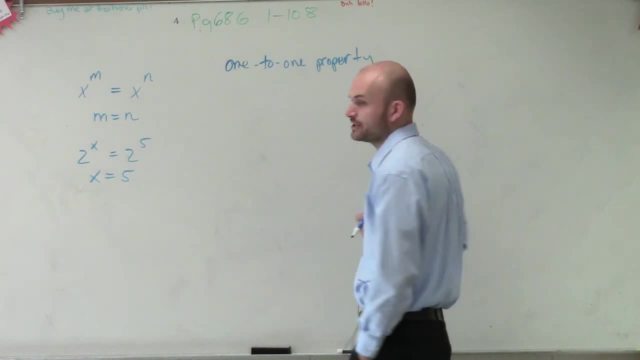 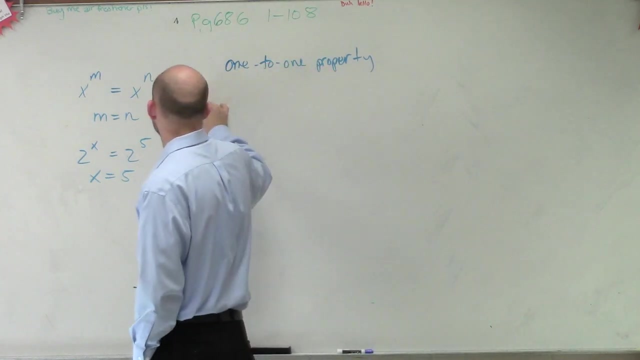 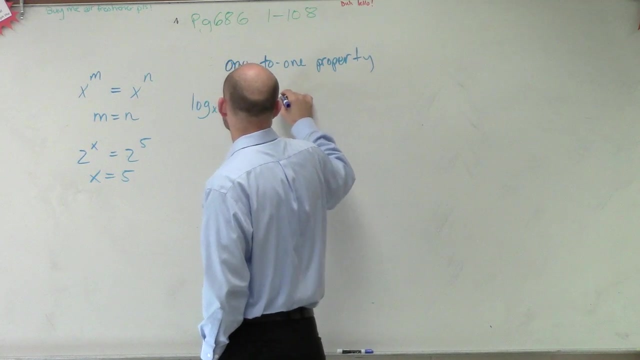 of use some numbers with that correct. So what I want to do is I want to explain. now let's use the one-to-one property for logarithms and see what it's going to look like. So if I had log base x of m equals log base x of n. 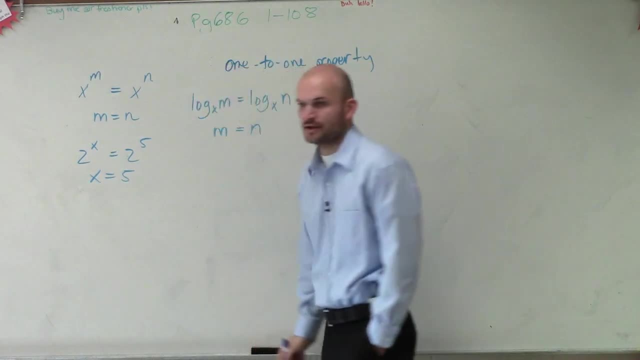 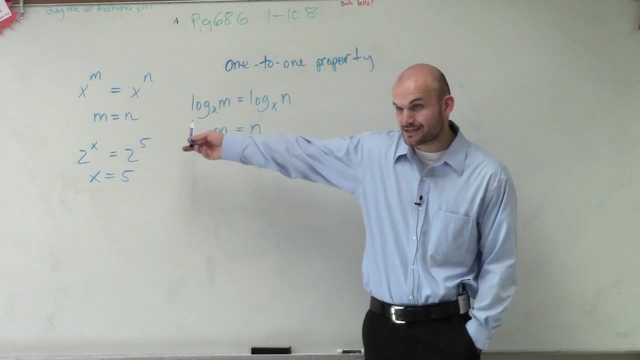 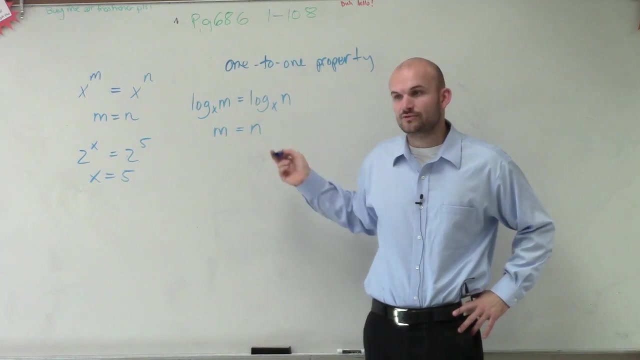 That means m equals n. So again, just like exponents, if I have a logarithm with a base x or with the same base equal to another logarithm, as long as they have the same base, what we're evaluating each logarithm for, are going to equal to each other. And let's take 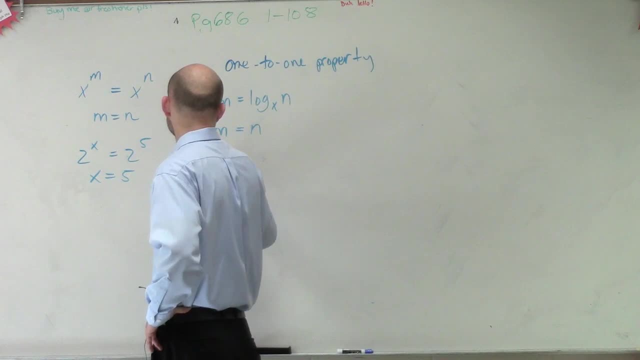 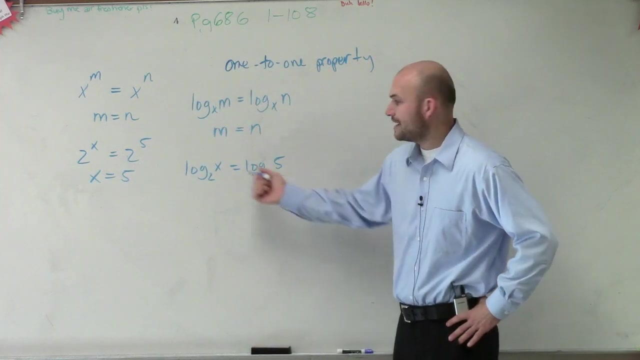 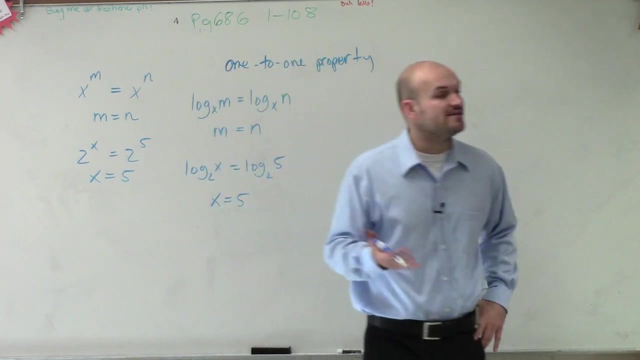 a look at that. If I had log base two of x equaled the log base two of five, then we We could say that x is going to equal 5.. So, again, a very important property that we can use is to make sure that we get our logarithms equal to one. 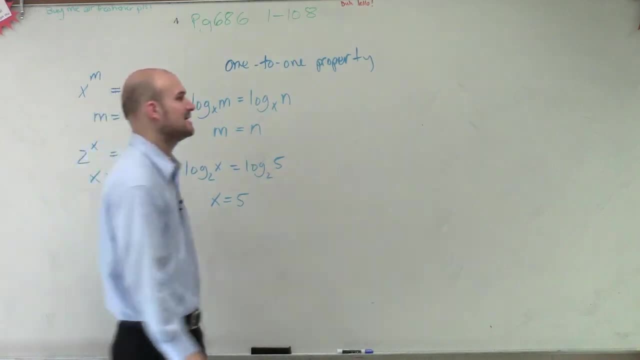 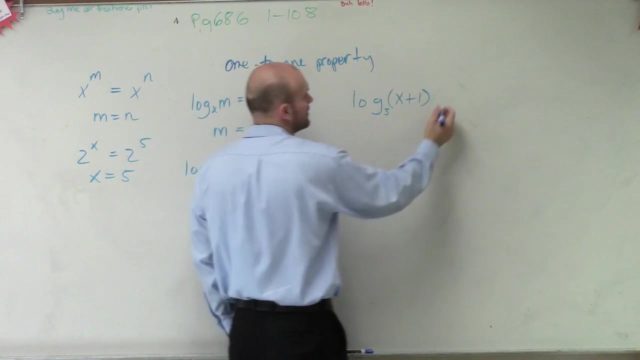 another. So let's go through a problem though, where a lot of students are going to make a mistake. So let's say I have an example of log of x plus 1. And let's use log base 5 minus log of base 5 of x. 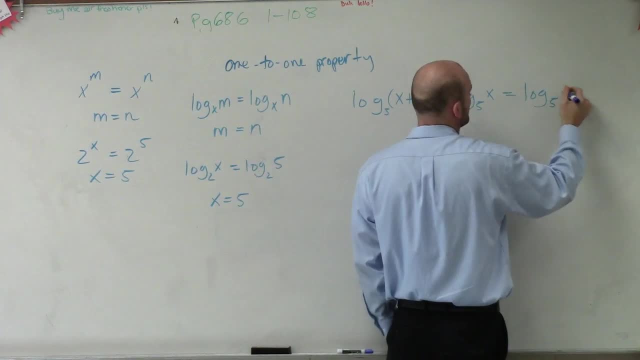 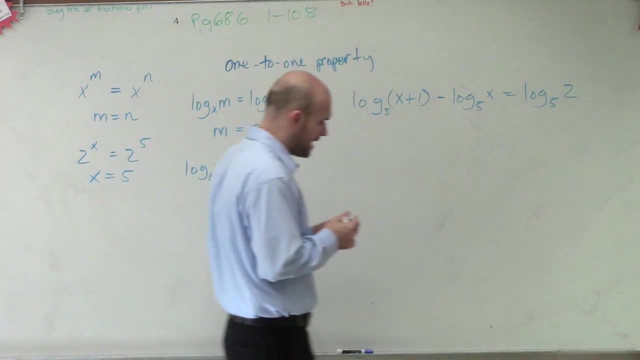 equals log of base 5 of 2.. So here's a very common problem that you guys might see that we're going to take a look at it Now. I put this problem up here because one of the most common misconceptions for a student. 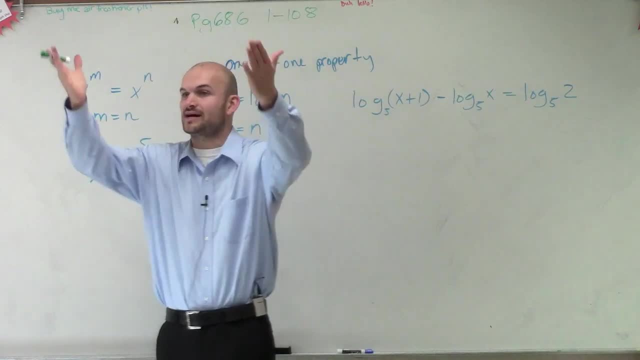 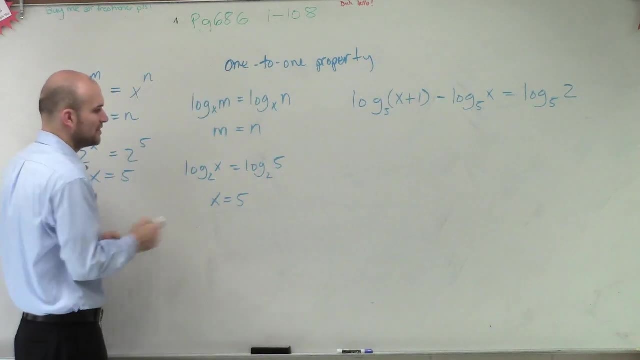 Marco, is you'd say, hey, I have a logarithm on both sides, so I have to then do what? Cancel them out. right, That makes sense. That's what I just taught you. Hey, when you have a logarithm, as long 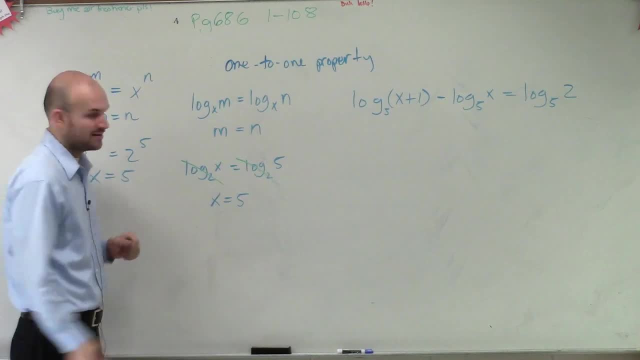 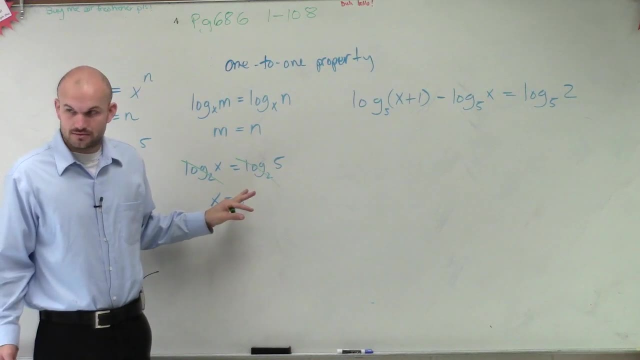 as they have the same base, which those do, we don't really need them. then We can just evaluate. But does this or does this look exactly like that? No way, No right. This is not. one logarithm equals another logarithm. 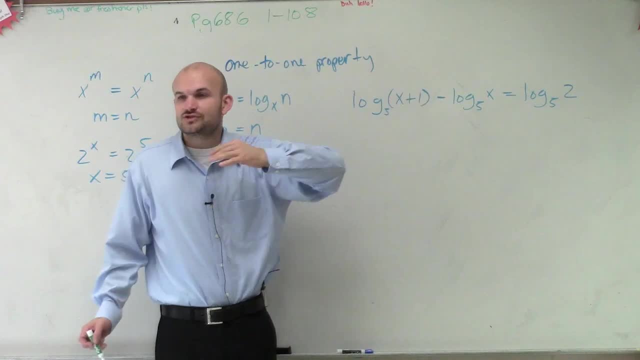 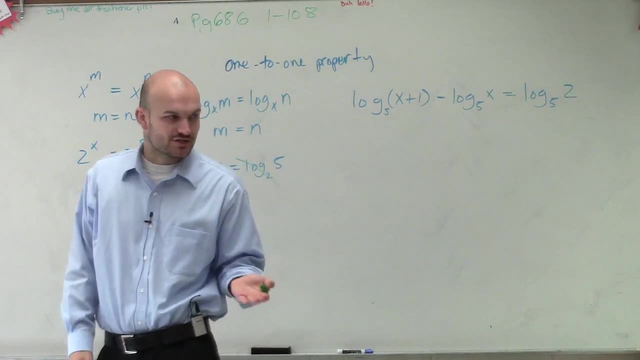 This is a logarithm minus another logarithm equals a logarithm, So we cannot just say: oh, eliminate the logarithms. Now, when we have a subtraction symbol- does anybody remember subtraction? When we subtract two logarithms, we can rewrite that as: 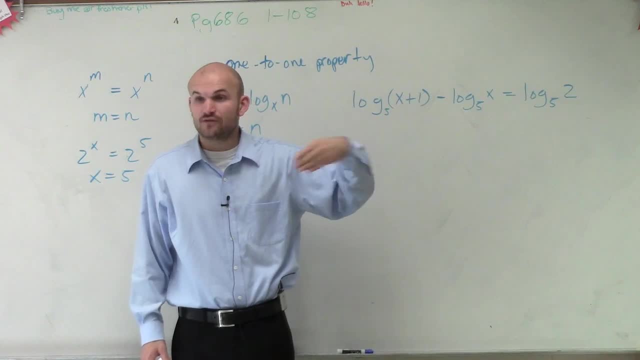 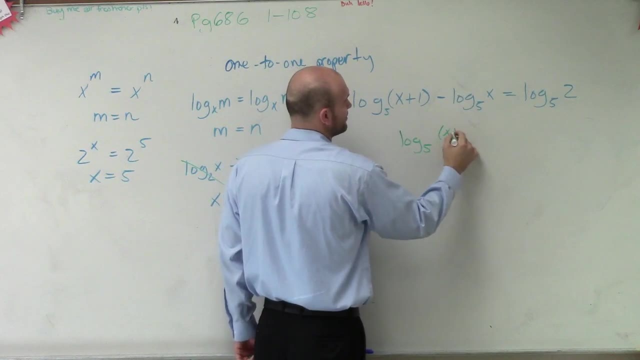 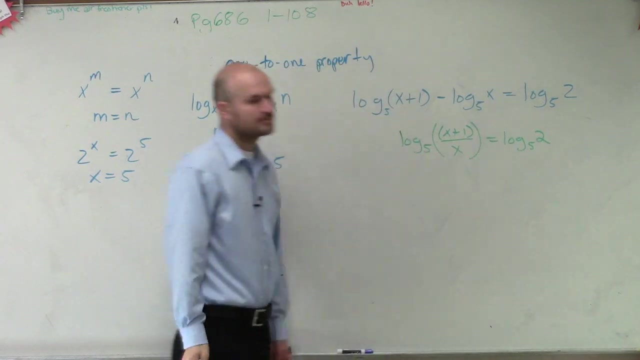 Divide. Divide As the division or the quotient of one logarithm. Yes, So I can rewrite this as log base: 5 of x plus 1 over x. Do you guys agree with me? That's what I talked about last class period. 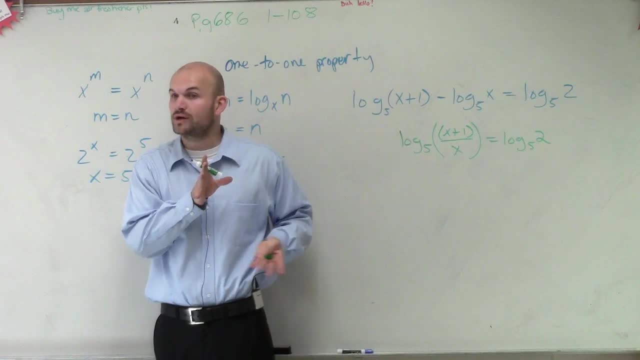 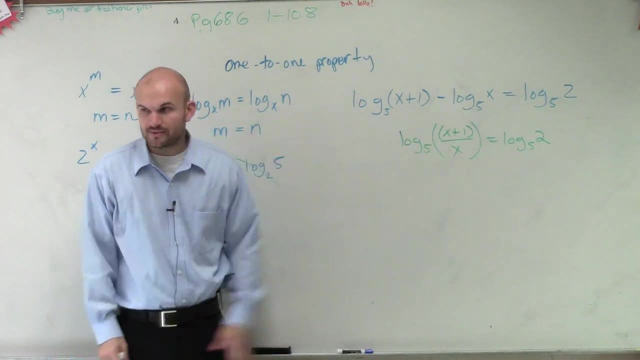 If you have the subtraction of two logarithms, you can rewrite it as the quotient of one logarithm, And that was what those little practice problems we did Condensing right. So now do we have a logarithm equal to another logarithm. 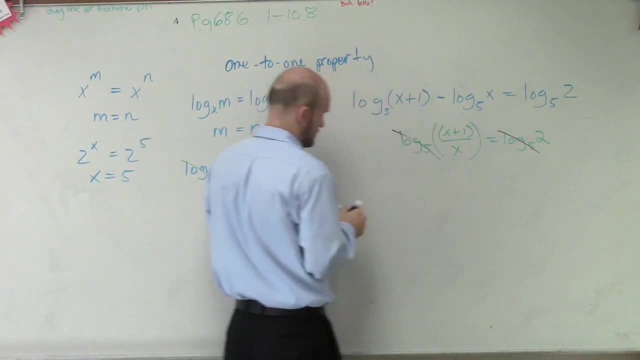 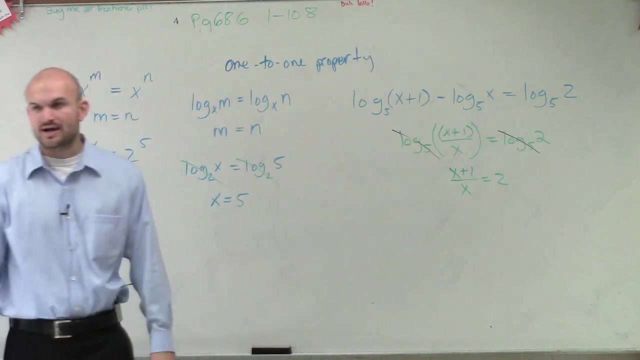 Yeah, and they have the same base. So now I have x plus 1 over x equals 2.. So now I need to learn how to solve this right. Well, remember, guys, we can get the x off the bottom by multiplying x on both sides. 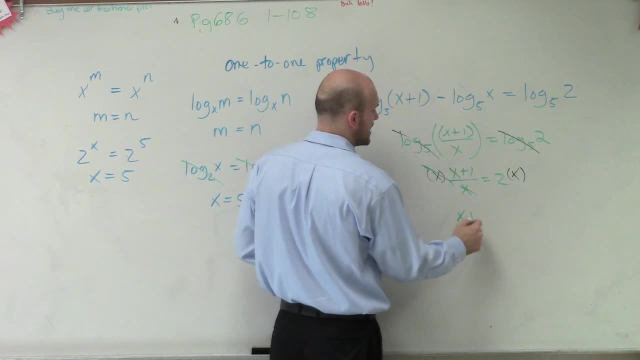 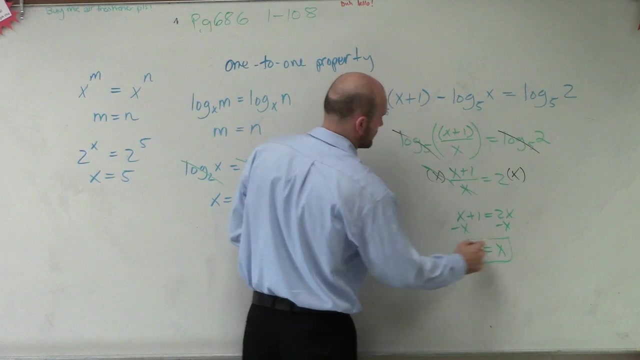 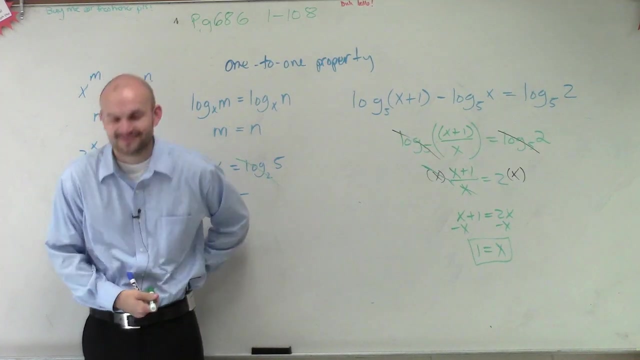 So therefore, I have x plus 1 equals 2x subtract x. subtract x: 1 equals x, And there you go. That's your final answer. OK, OK, That's it.